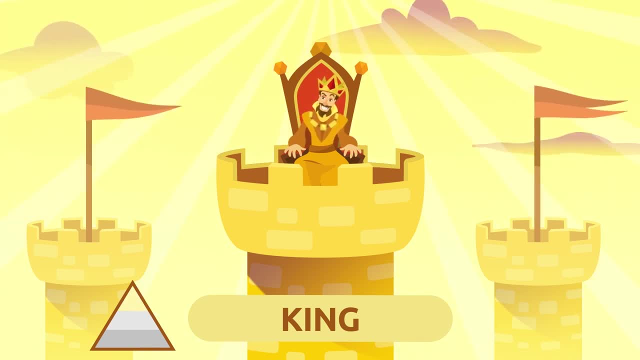 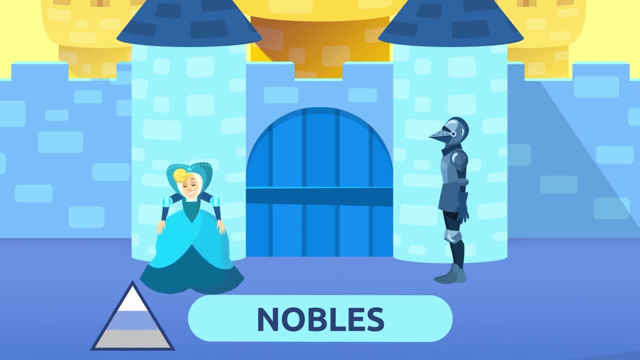 before had the power and ruled over the land with clerical consent. Right below the king and the clergy were the nobles. They ruled over the lands allocated to them by the king in exchange for swearing allegiance and defending the country during warfare. 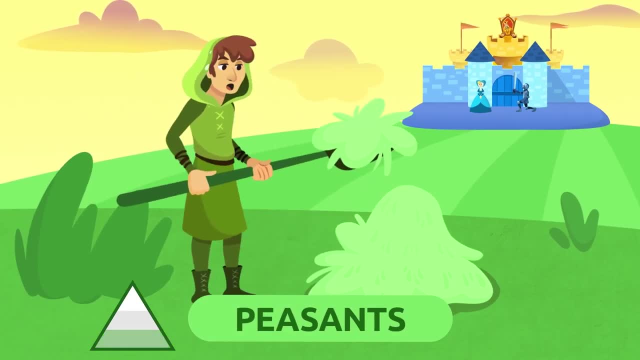 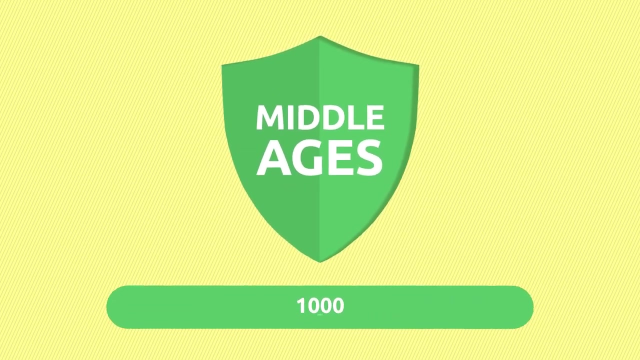 Nobles had authority over peasants and vassals, known as serfs, who worked the land and lived there. They worked for protection. In exchange, peasants paid high taxes to their lords. As we said before, the Middle Ages lasted more than 1,000 years. That's why we divide. 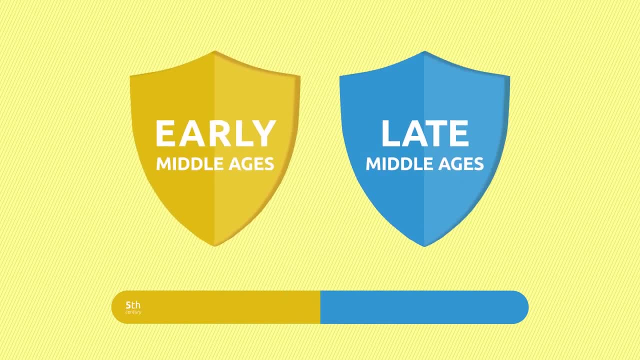 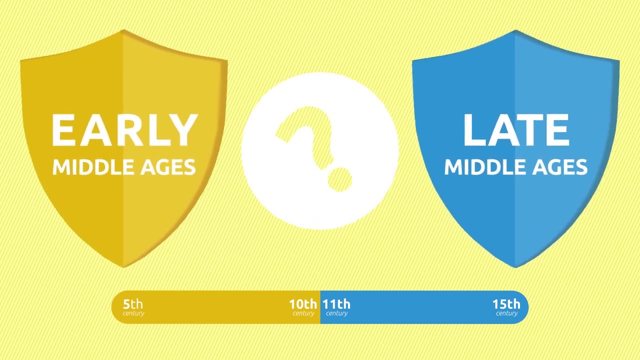 this period in two phases: the Early Middle Ages, from the 5th to the 10th century, and the Late Middle Ages, from the 11th to the 15th century. What's the difference about each phase? During the Early Middle Ages, the nobility 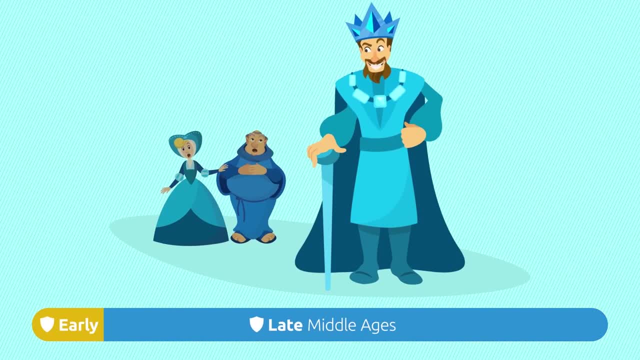 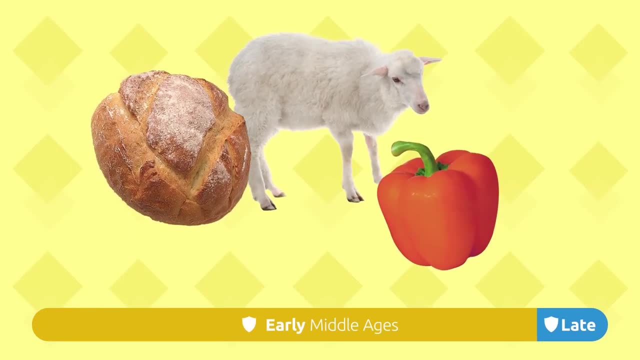 and the clergy had a lot of power. In contrast, during the Late Middle Ages, the monarchy takes power back. During the Middle Ages, agricultural and cattle-raising were solely a means of sustenance, that is to say to feed the people. By contrast, during the Late 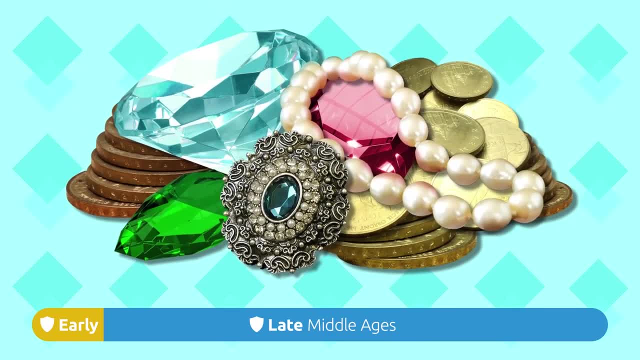 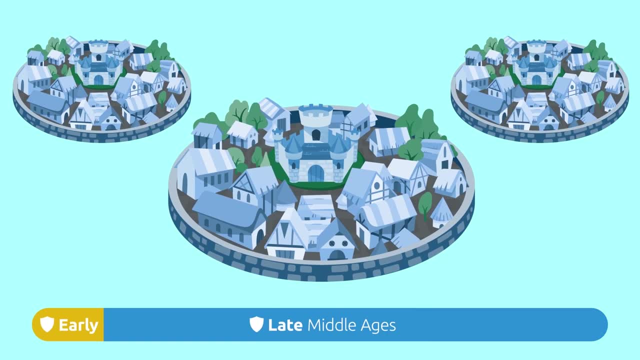 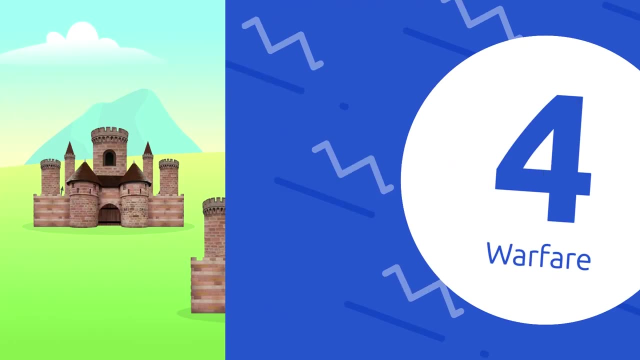 Middle Ages there's an increase in production and commercial activity, While in the Early Middle Ages people lived on fiefs. During the Late Middle Ages there's a resurgence of the cities that become the new economic centers. During the Middle Ages, warfare was very common. The importance of knights derives from this. 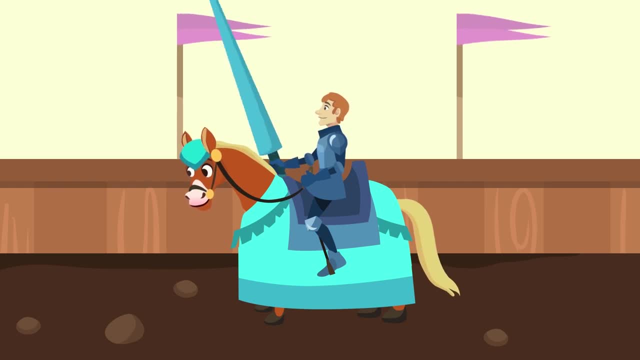 fact, as they played a key role defending their king and nobles, Knights were taught fighting skills and were trained with all sorts of weapons. They wore a heavy armor and a helmet which protected them. Many knights were members of the gentry. Apart from warfare, there was 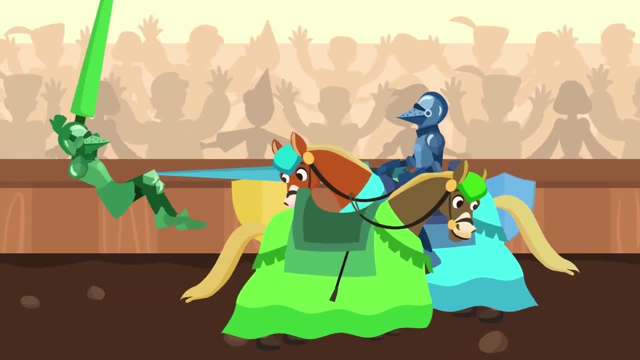 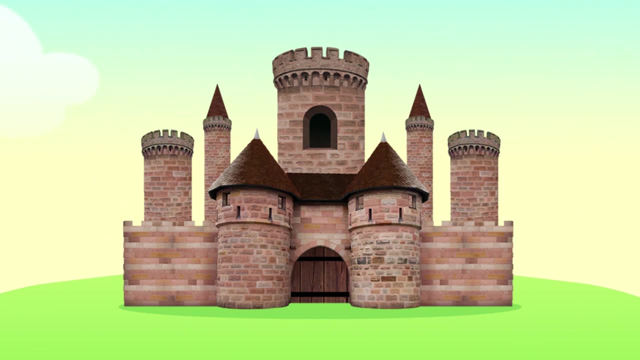 a lot of fighting Knights also participated in tournaments and jouts, risking their reputation and prestige. Have you ever seen a medieval castle? Castles were fortified structures typically built in the Middle Ages. They were situated on high ground, which made defending the territory.